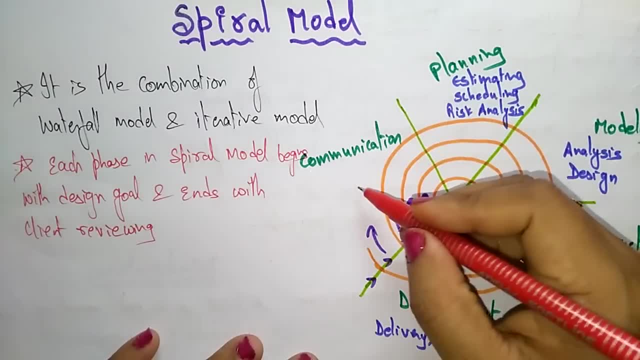 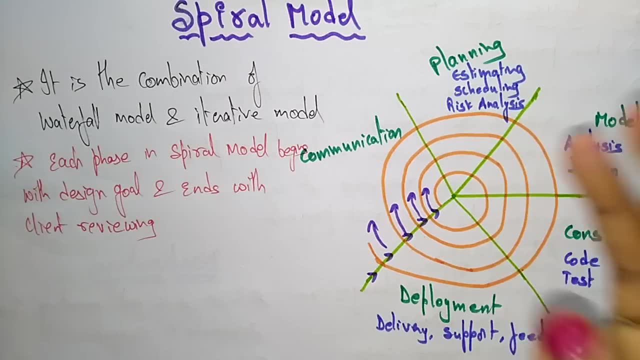 modeling or construction. so here different five phases- i am taking communication, planning, modeling, construction and deployment. so here in each phase in the spiral model it begins with the design goal and ends with the client reviewing. so using spiral model, software is developed in a series of incremental release. so the main thing is here: uh, software is developed. 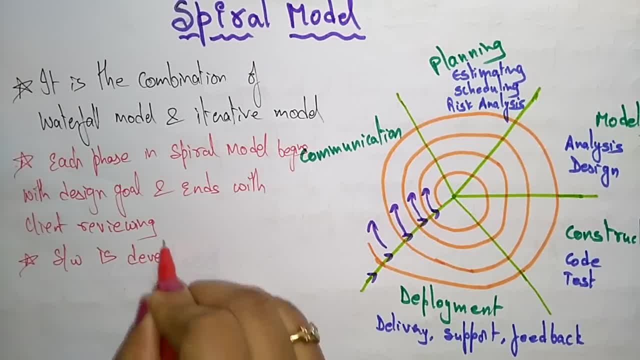 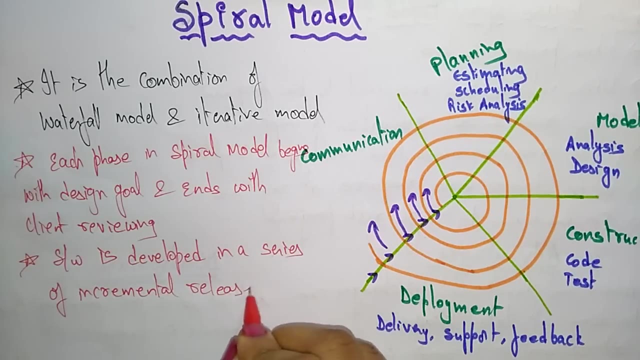 software is developed in a series of always. it is to be incremented in a series of release, series of incremental release, incremental releases. so here a spiral by uh model is divided into a framework activities, also called as a task region. so these are different task regions. so here you can see. 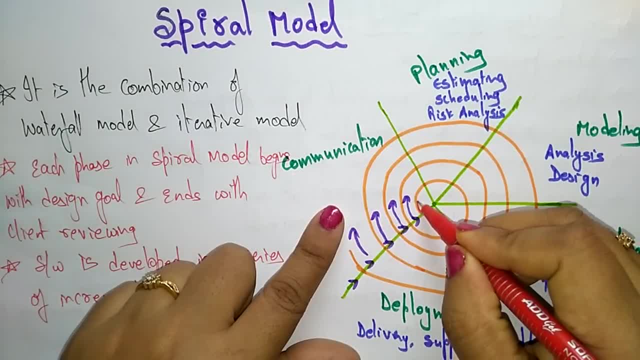 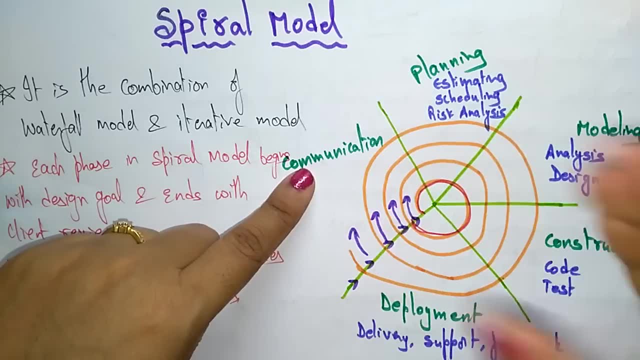 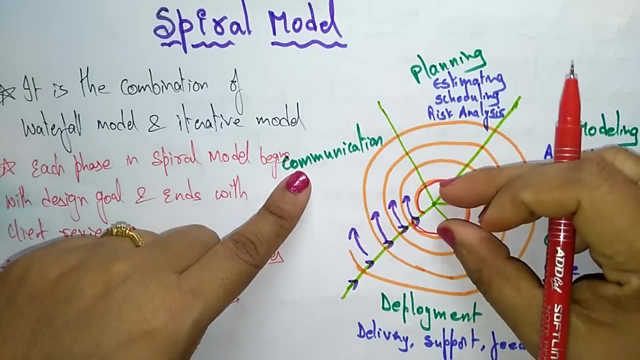 this is a spiral starts from here, so this comes to one phase, so up to here this is one phase. so uh means one task. i'm talking about the task. so a spiral model is divided into a framework activities, also called as task regions. this is one task region and next this is another task region. 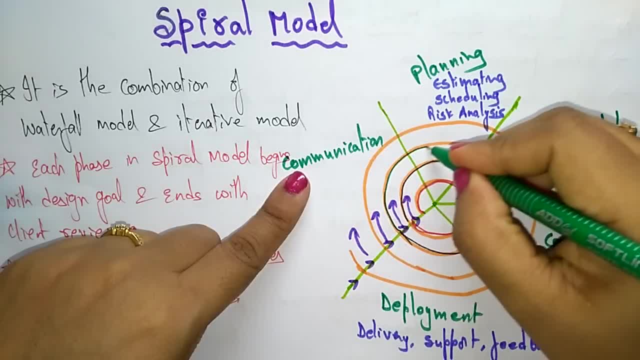 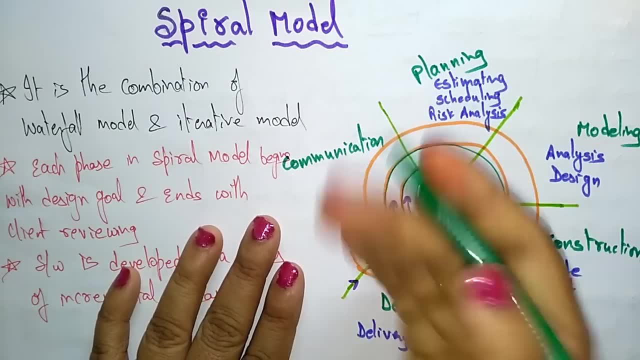 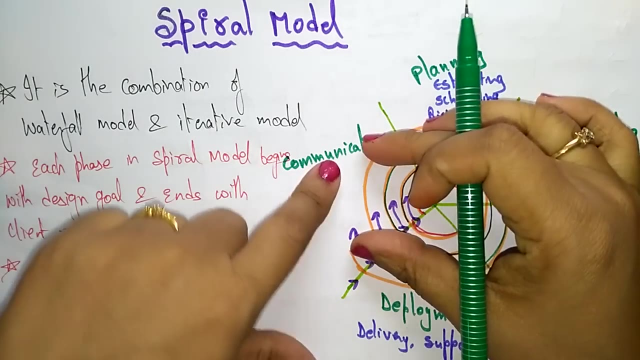 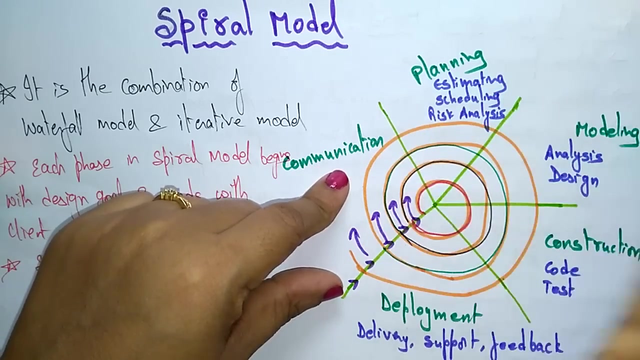 okay, and next this is another task region, like that. these are the different task regions that are present in the spiral. so first stage is a communication, so a communication it come. a communication between the customer and developer is starting here. so first we discuss the project with the customer. so what are the requirements they want? that is a communication, they are just 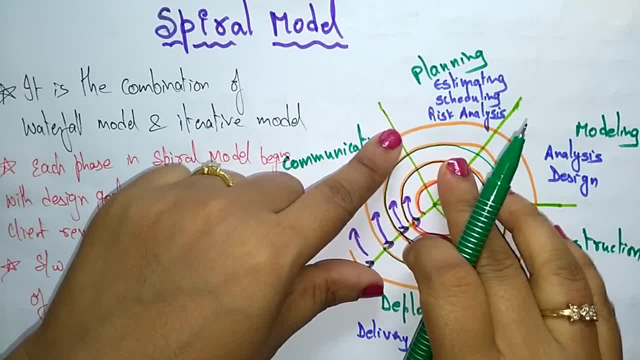 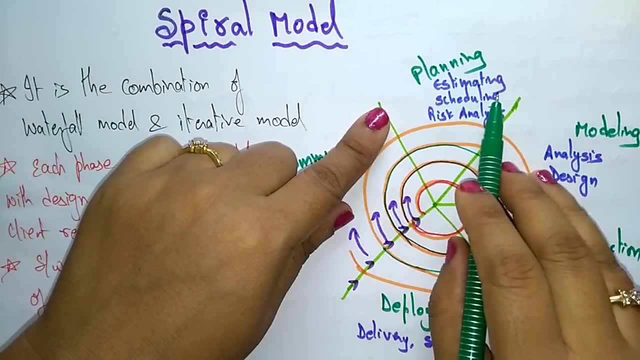 talking so and next they are planning means the developer has to plan whenever they take the project. so the developer has to plan the project. and then the developer has to plan the project. so in the planning comes for uh, it's nothing but estimating of the project, scheduling the project. 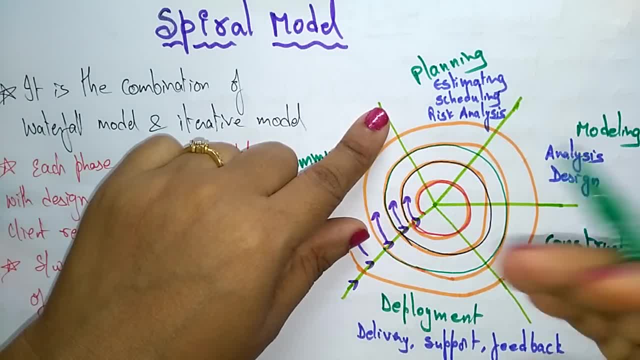 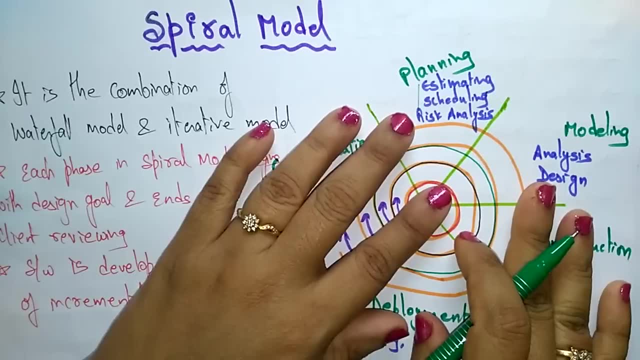 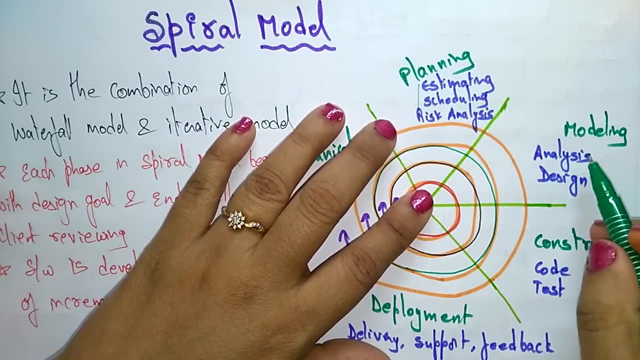 and any risk analysis. risk were undertaken while we developing the project. so those are all comes under the planning. so after planning we have to model means the design. once the documentation is ready, we have to design in the pictorial representative. that is the modeling. so in the 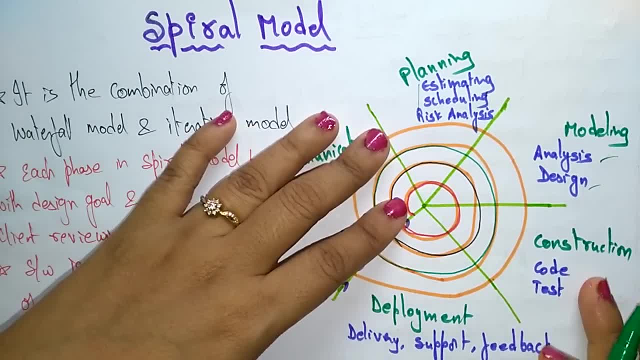 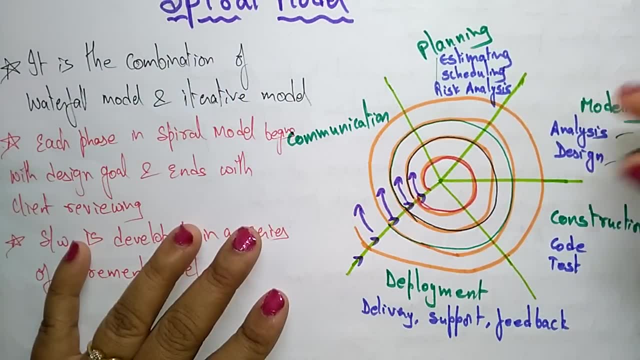 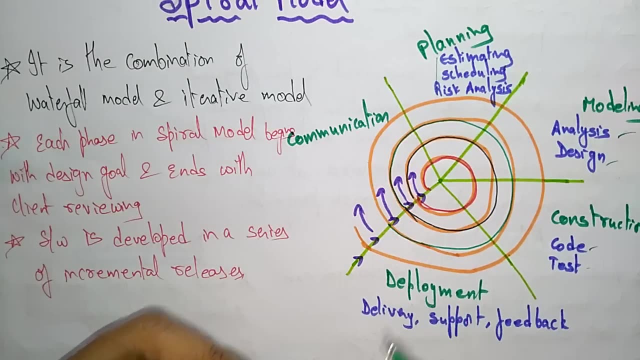 modeling. you come across with the analysis phase and the design phase. so, okay, my modeling will be over. means i- whatever the documentation is there that will be represented in a diagrammatic form. after that i have to construct. means the construction comes under code and test. means i have to write the code for that project. and after writing the code i have 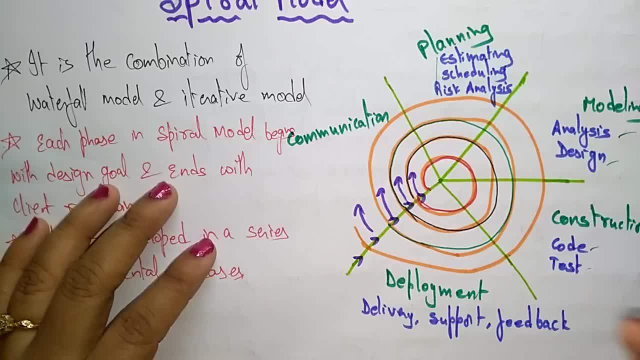 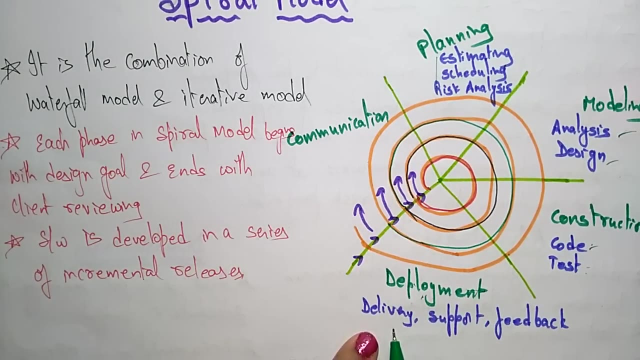 to test whether any uh means is a product is success or not. i have to test. okay, that is a code and test will comes under the construction phase. after construction, the project is ready, so i have. that is a deployment phase. so in the deployment phase you came across the delivery of project and 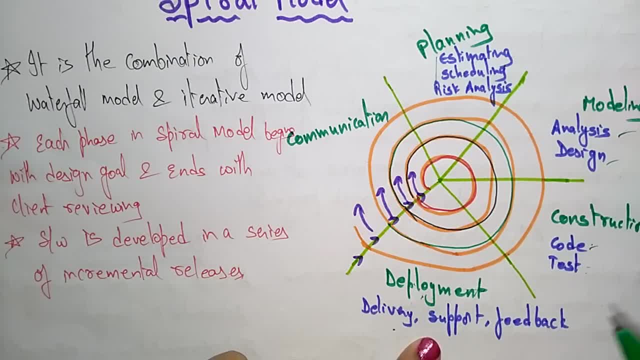 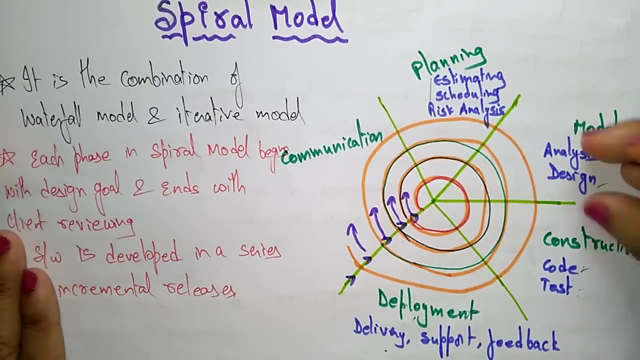 support if there any need to the customer means regarding the project. if there is any support requirement, you have to provide that. the developers has to provide the support and the feedbacks from the customers. so these are all the different phases. so, whatever the model you have taken, these phases will come: planning, modeling, construction, deployment, communication, so whatever. 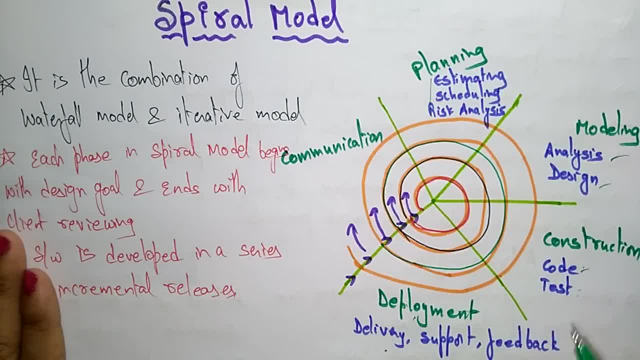 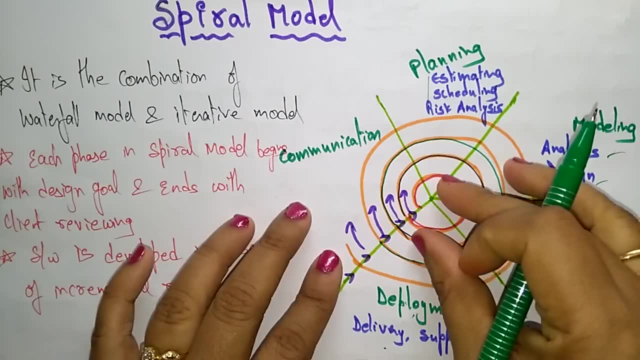 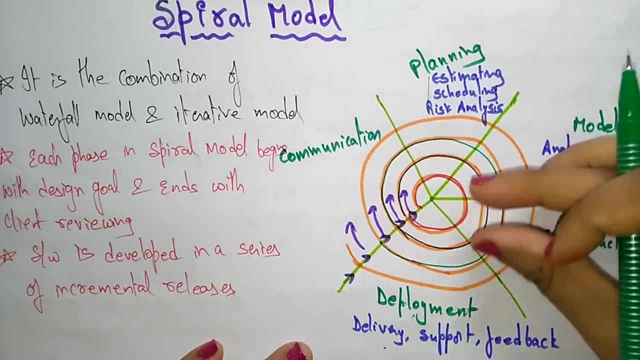 the model you have taken, these phases will come. but here, in the spiral model, uh, the software is developed in a series of incremental release means once, once it will be released, after another increment will be there. so it is divided into frameworks. the main thing is here the task will be, uh, task regions will be there. so these are the different task regions. 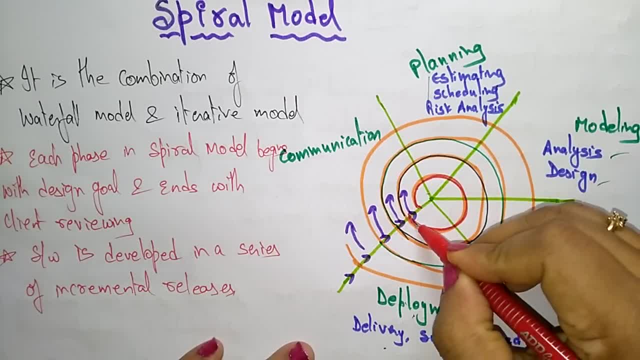 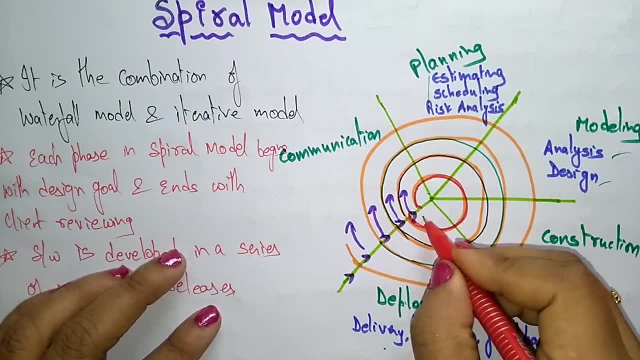 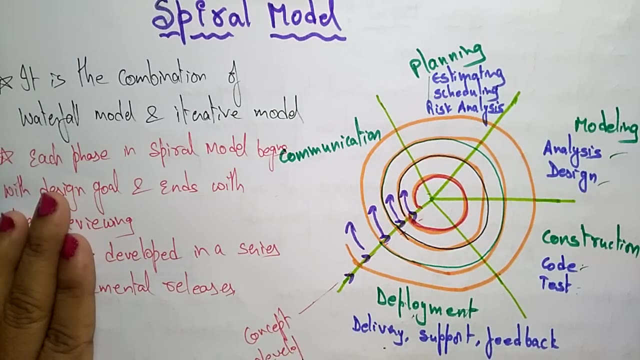 so if you take the first task region, this is one task region. so this task region, uh, it explains the concept development. so this indicates the concept development. so in the right circle it's indicates the concept development. so the first, most inner circle means here we are developing the concept. 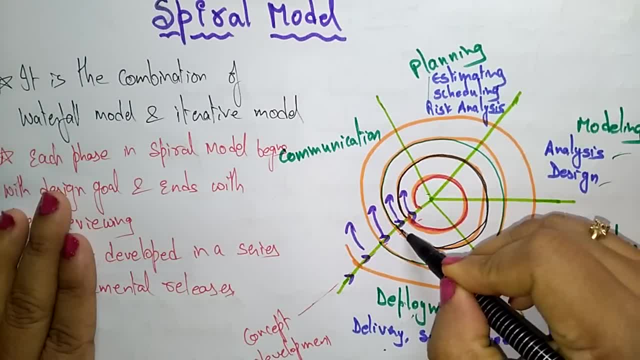 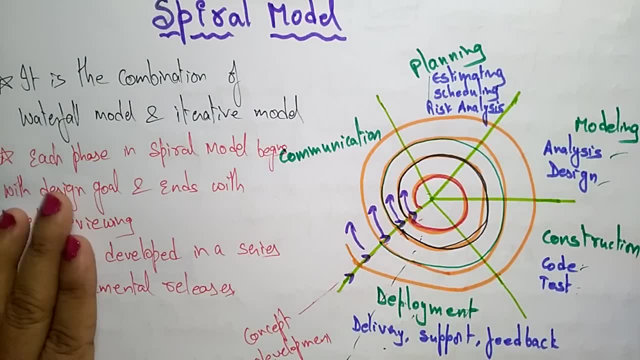 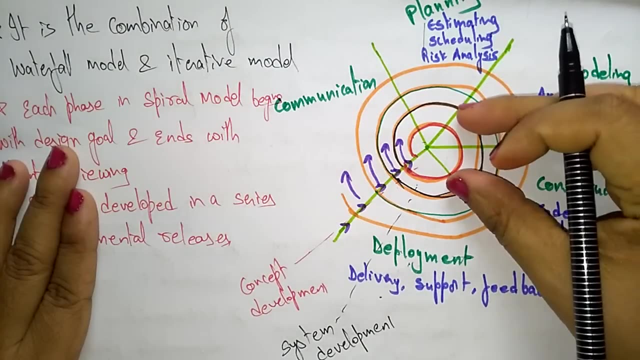 so after that, so in the next circle, so this next spiral. so this comes under this, uh, system development, this is a concept development and this comes to the system development, system development to be developed. first the concept is developing, okay, concept is ready. then you have to prepare. 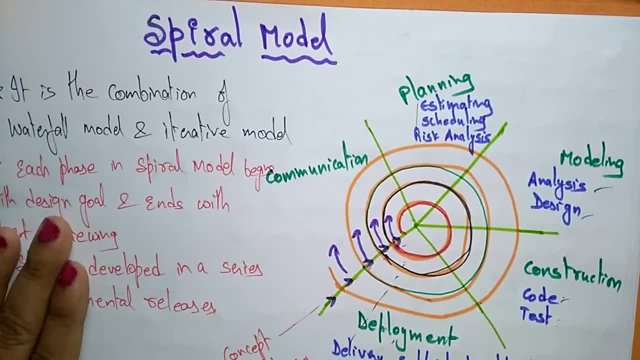 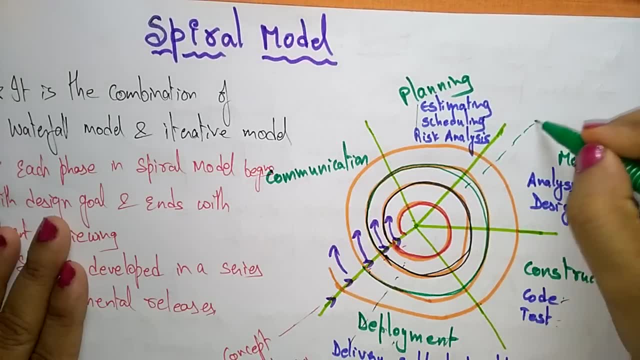 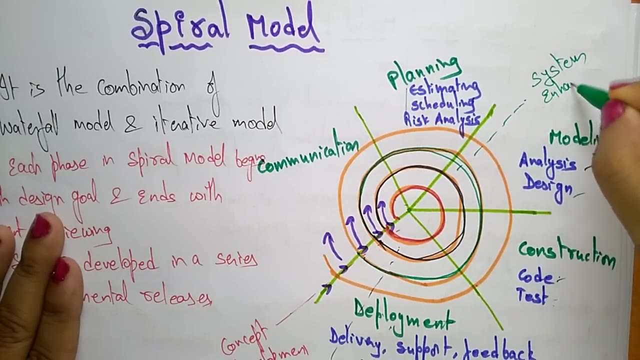 for the system. so system development. so after that, this is the uh next task region is this is the next task region, so this task region explains about the system enhancement. if there any enhancement required, that will be uh done here. system enhancement: so after system was developed, the system has to be an enhancement in this part. and the last thing, that is the 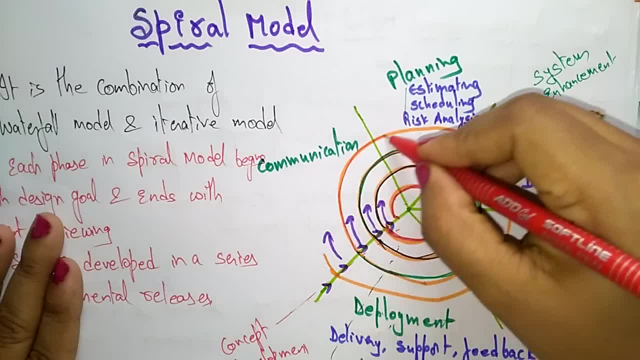 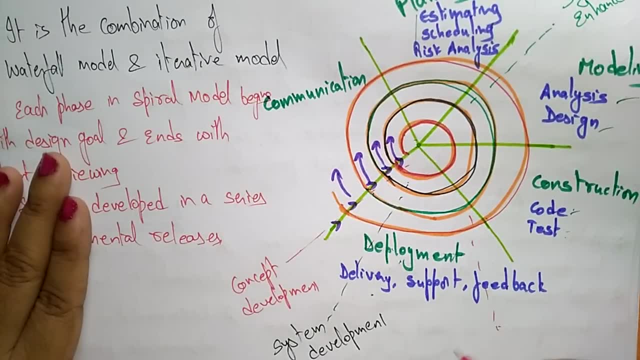 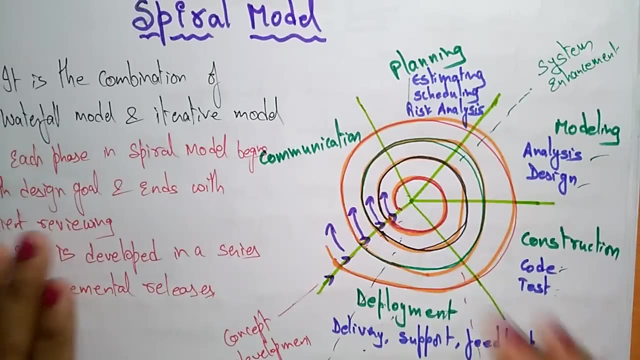 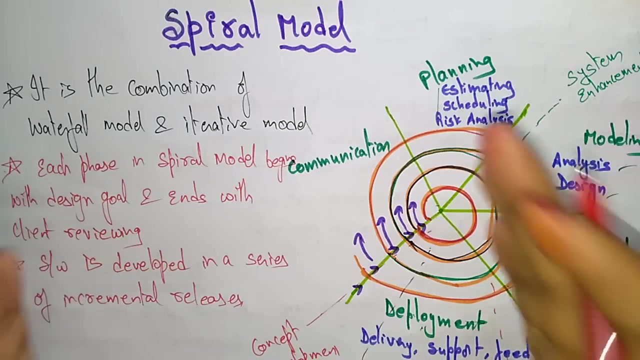 here i'm taking. this is another spiral, so this spiral indicates the system maintenance, system maintenance. so these are all the different tasks that are presented in this pile. so this is about the spiral model. so, whatever the model you have taken, everything will be planning, modeling, constructing, deployment and communication. so the main difference between the 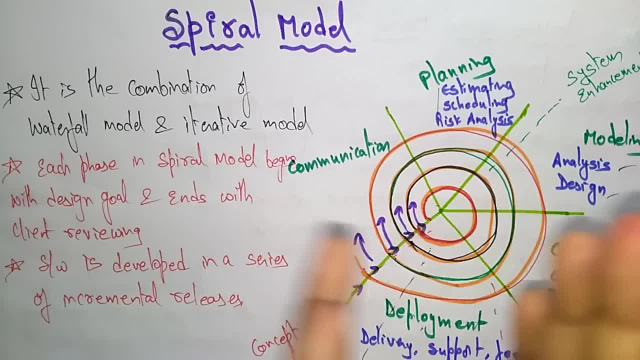 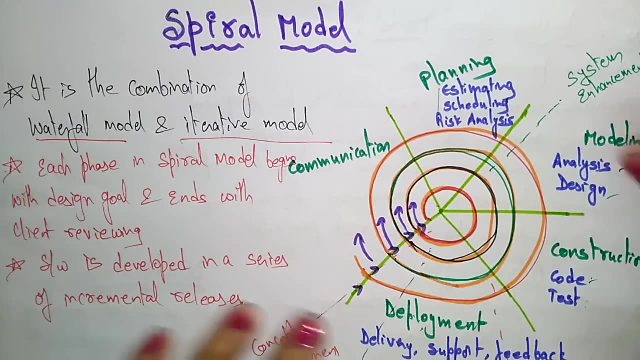 models or means, while we are following the sequence method, while we are following the iterative method, while we are- for what? uh, following what type of methods to develop a project. so the spiral is a combination of both waterfall model and the iterative model. now let us see why. 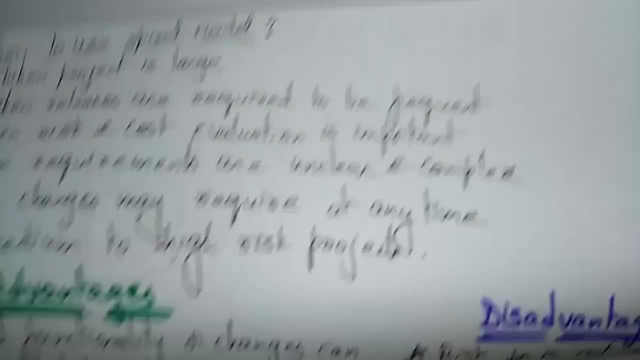 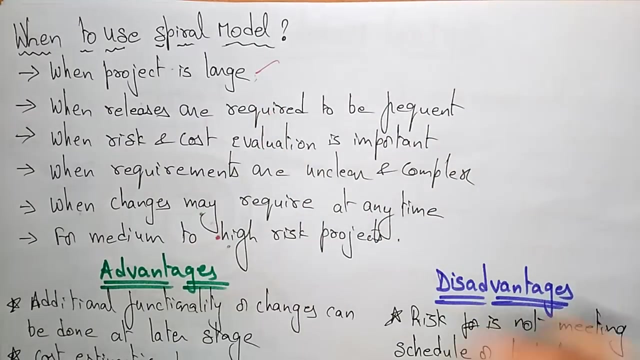 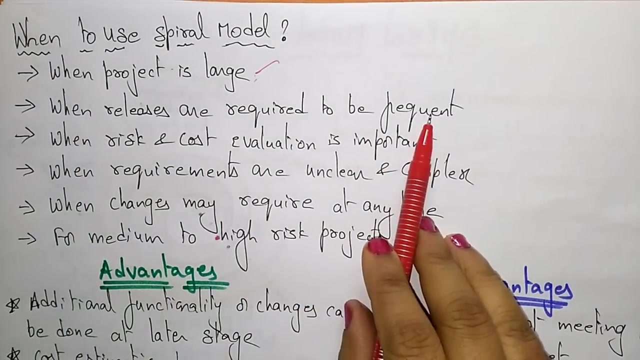 uh, when to use this spiral model, when we are going to use a spiral model. so when you are discussing- uh, dealing with the large projects, go for the spiral model. the best way is to go for the spiral model if you are dealing with the large projects, when releases are required to be frequented. 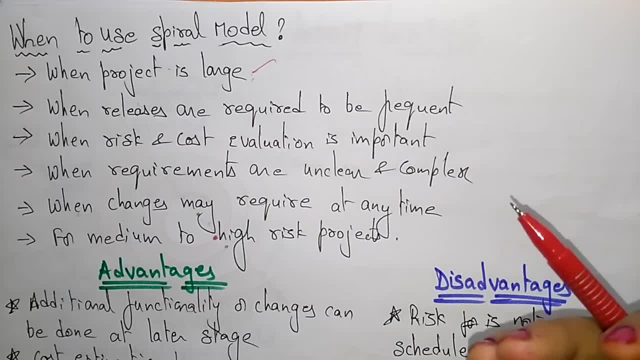 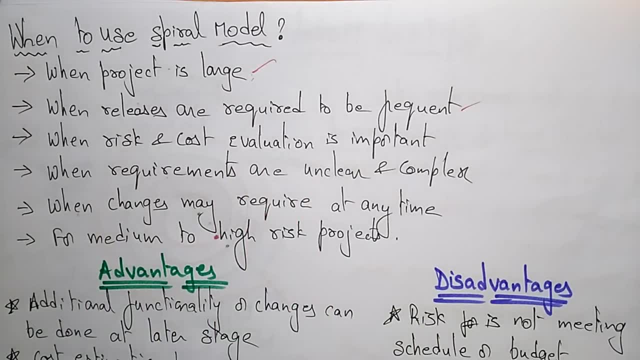 uh, so so far? uh, frequently, if the release is required, then it's better to go for this parallel model. so if there is any risk and cost evaluation is there, means, if you want to calculate the risk and cost evaluation for every time, then it's better to go for the spiral model. the spiral model is: 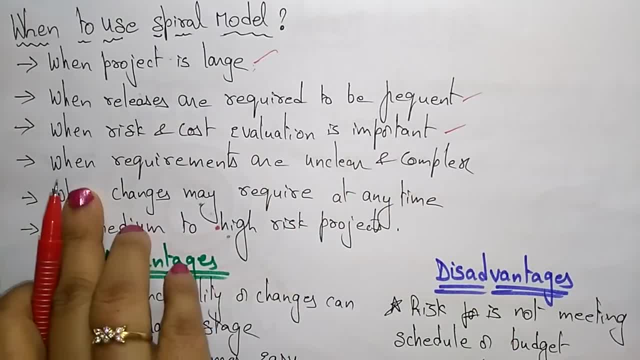 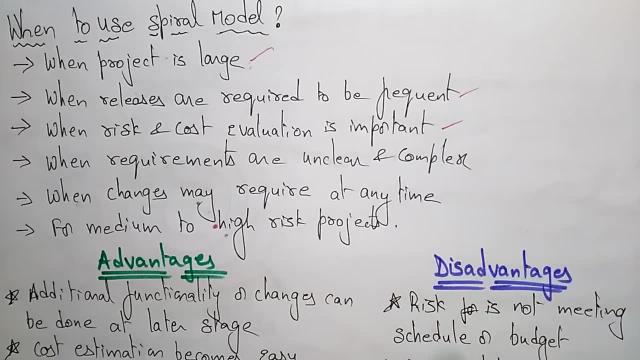 used when risk and cost evaluation is important. so when requirements are unclear and the complex means the requirements, whatever the customer has given that were not clear, and if those requirements are complex seems to be complex, then it's better go for the spiral model means in the spiral model every it's. just we are developing a series of incremental release, so whenever you 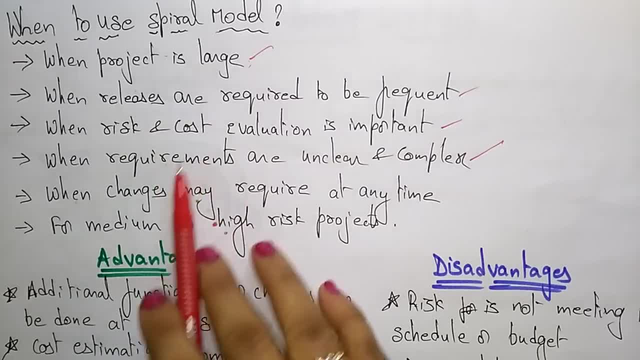 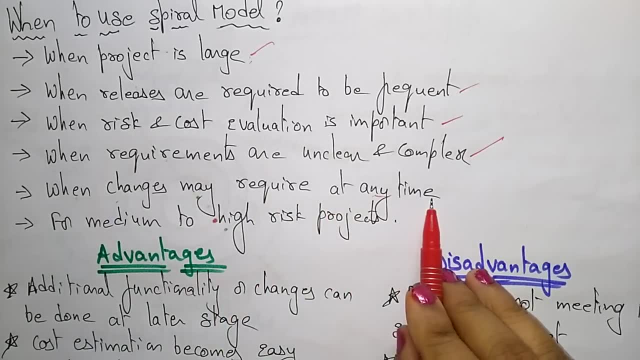 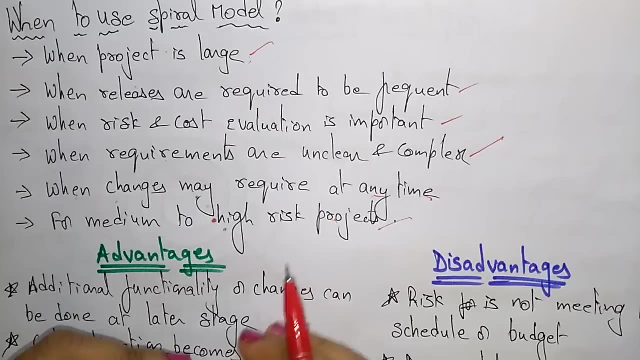 want you, you can add the features to that. so if when requirements are unclear and complex, better to go for the spiral model, so when changes may require at any time, then go for the spiral model for medium to high risk projects. whenever you are adding the medium projects to adding the 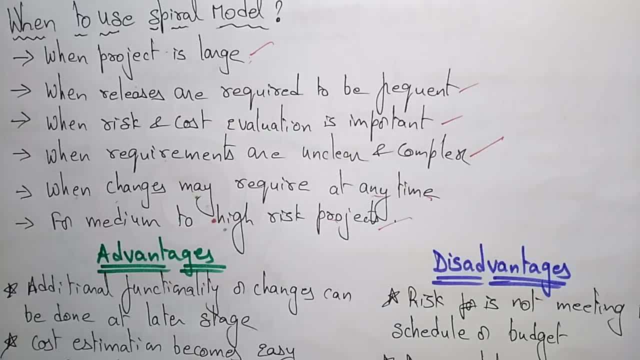 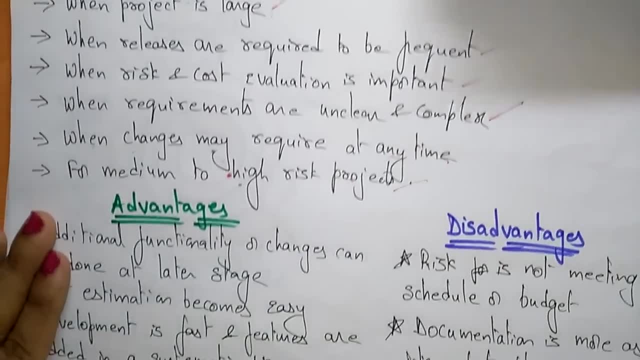 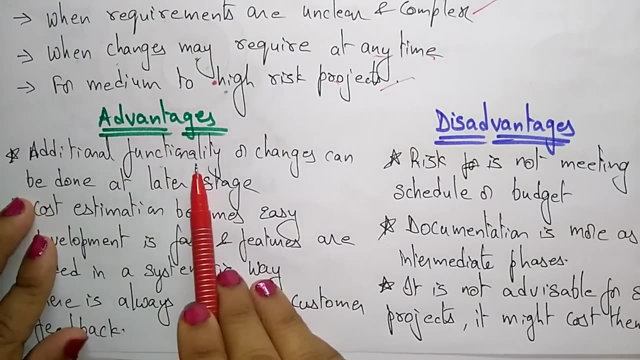 features and you making it a high risk project means it seems to be high risk project, then you can prefer spiral model. so in this cases we will go for the spiral model. now, coming to the advantages and disadvantages of using this spiral, let's see the advantage: additional functionality or changes can be done at later stages. so whatever the functionalities, 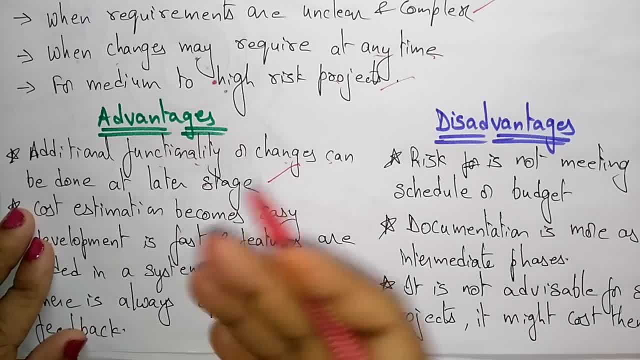 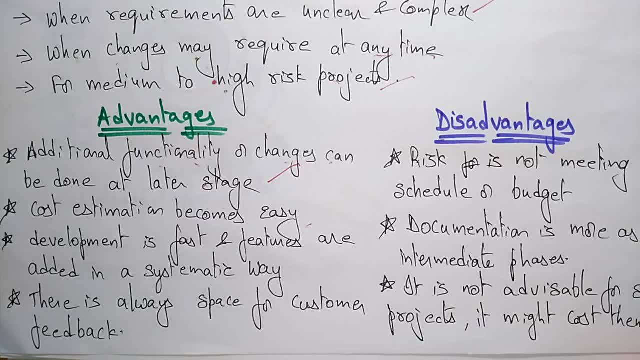 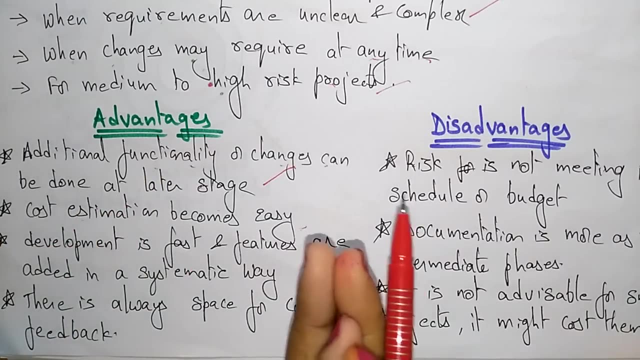 and whatever the changes that you need to require in the project. you can then at a later stage also, cost estimation becomes easy, okay, so in the each stage you can maintain the cost estimation. means this task, this will be the cost, means the system maintenance cost, system development, cost concept development cost. so like that, system enhancement cost, so cost estimation. 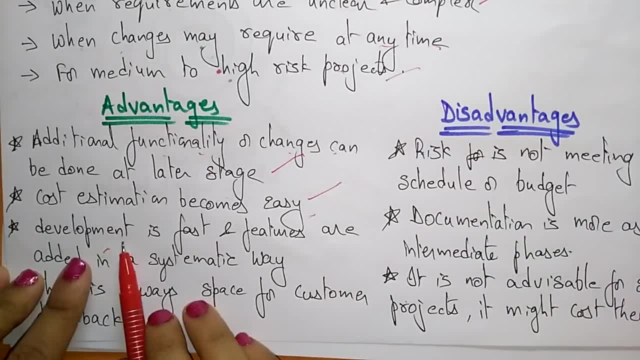 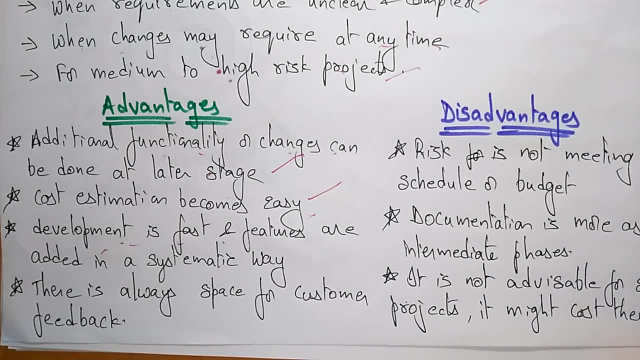 becomes easy in spiral model. so in spiral model development is fast and features are added in a systematic way. so always the features are added in a systematic way in spiral there is always space for customers feedback. so whatever the customers wants to give, the feedback you can. they can give. frequently means if they want, at any time they can give. so there is a space. 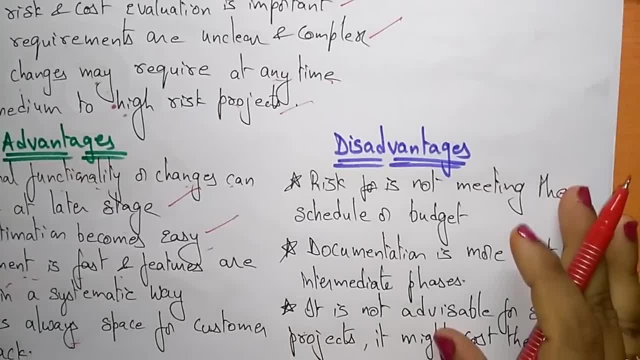 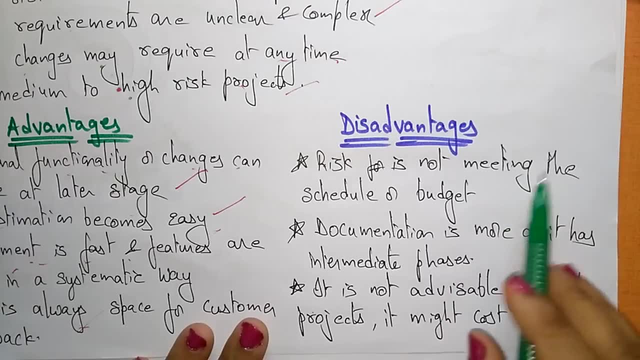 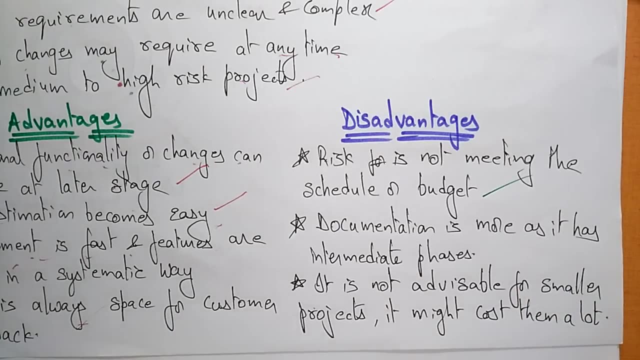 for customers feedback in spiral model. now let us see the disadvantages. the disadvantages is of using the spiral is risk is not meeting the schedule or a budget and the documentation is more as it has intermediate phases, so they should. in intermediate phases, we have to write more documentation to make. 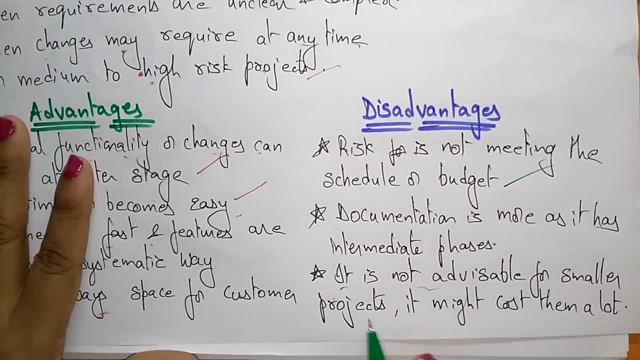 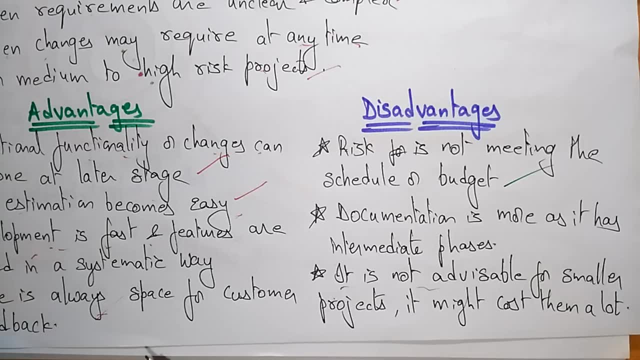 the each phase clear. it is a very important thing to keep in mind when you are designing a project- is not advisable for smaller project projects. it might cost them a lot. so I already said it's better to go for. if you are using this large projects, you can go for the spiral model. so it is not that much. 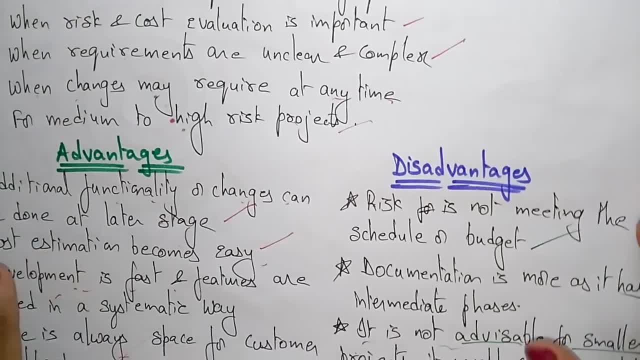 of suitable to the smaller project. so these are the advantages and disadvantages of using spiral model. thank you.